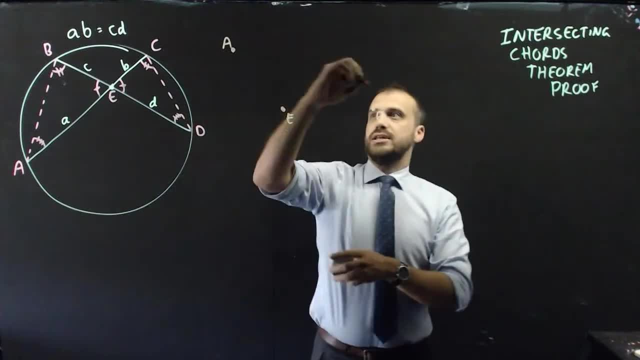 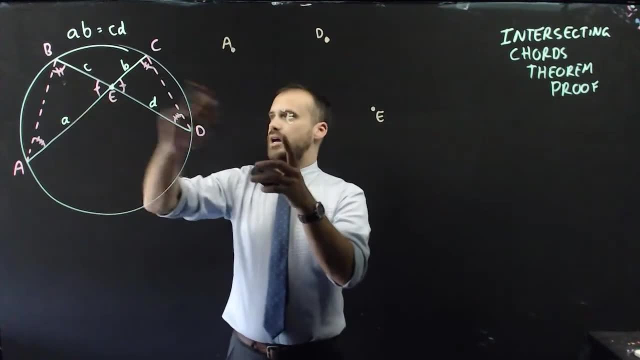 which means that over this triangle, D is the three dashes, So I'm going to put D there. This is going to make sense in a minute, I think. Okay, So we have A and E and then lining up with B here. 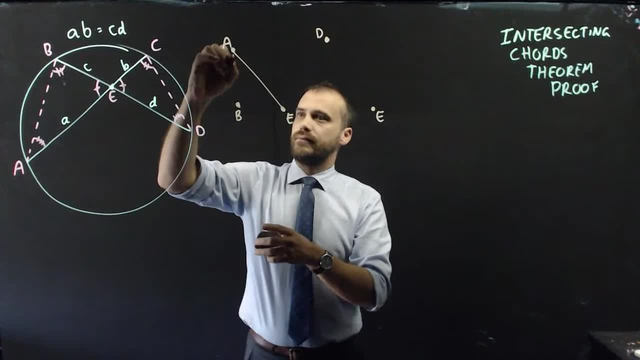 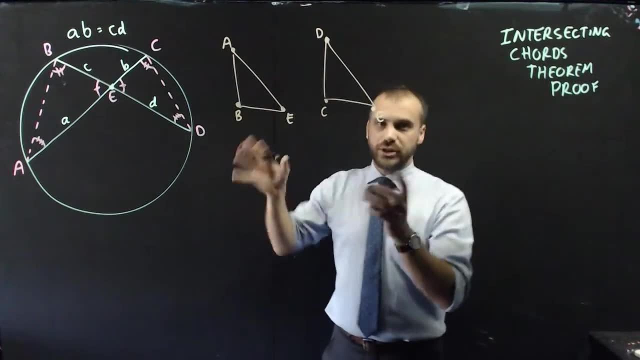 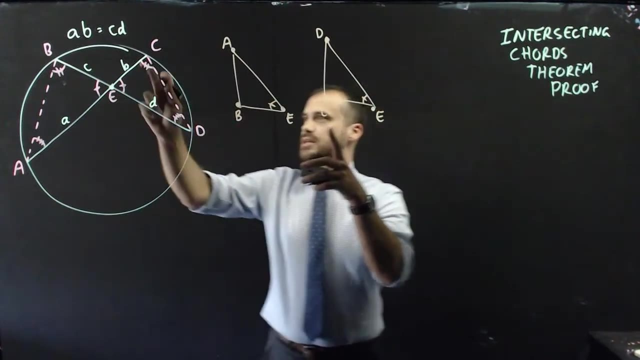 Okay, Okay, And obviously this one has C there. Now I do need to make sure I've drawn these triangles correctly. Now E has this one here. E has that one there. Now, from E to C, C has the like double dot one there. 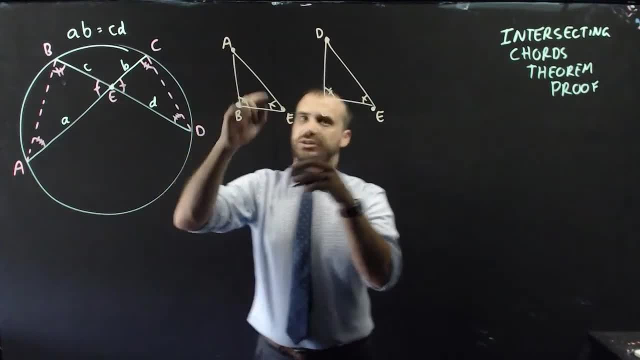 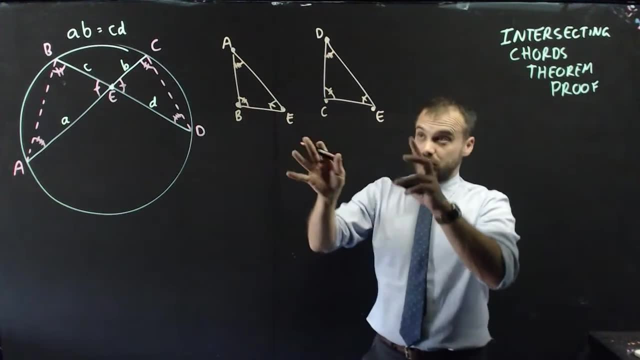 and B has the double dash, double dash, double dash. And then A has the triple dash and D has the triple dash. Now, They're not the same size. I've drawn them about the same size. They're not the same size. One's bigger and smaller than the other. 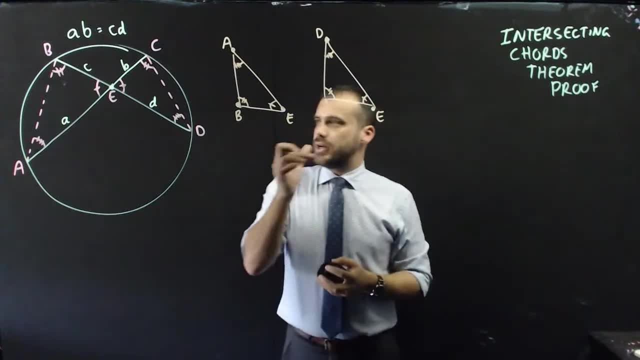 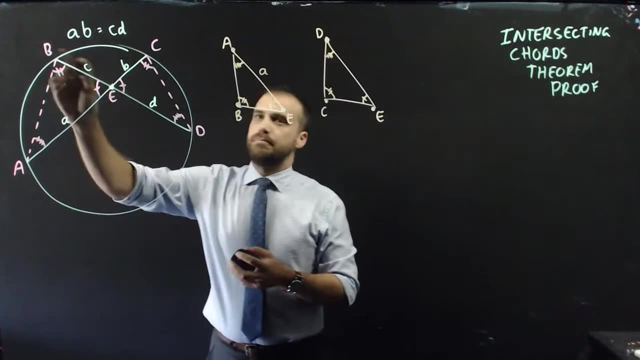 But they are similar because all their angles are the same. Alright, now let's label these things here: A to E, that's my lowercase a. E to B, that's my lowercase c. Okay, and then E to D, that's D. 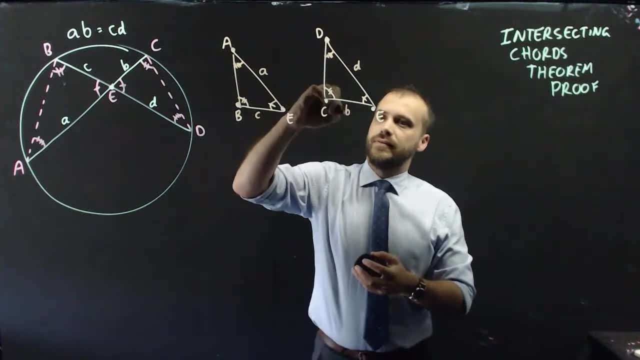 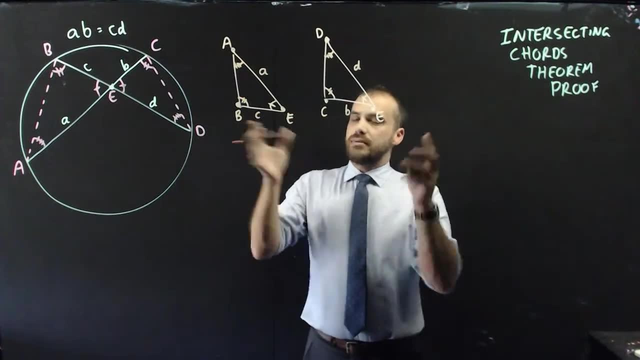 And E to C, E to C, that's B. Now, this is kind of an optional step here, but I really need to show you what's going on. Alright, so what we can say, because these triangles are similar, is that the ratio of this side to this side, C to B. 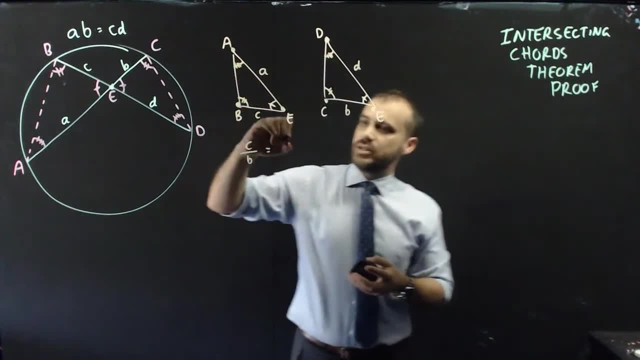 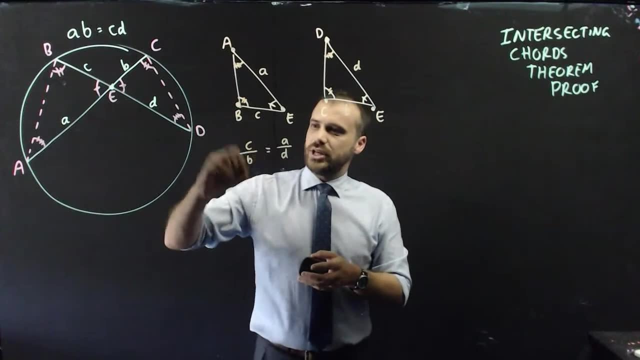 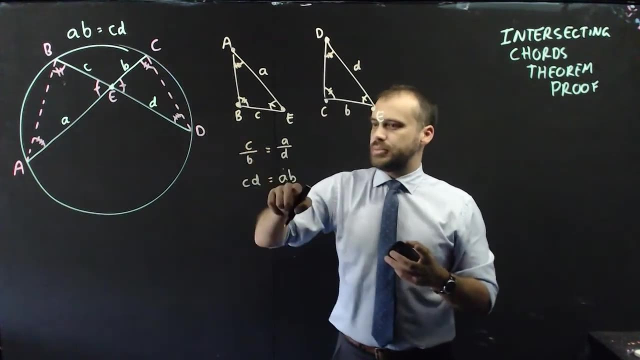 is going to be equal to the ratio of this side to this side, A to D, Because they're similar. Alright, if that's true, we can rearrange that to say that AB equals CD, AB equals CD. That snuck up on us. That's the proof. That's it Done. 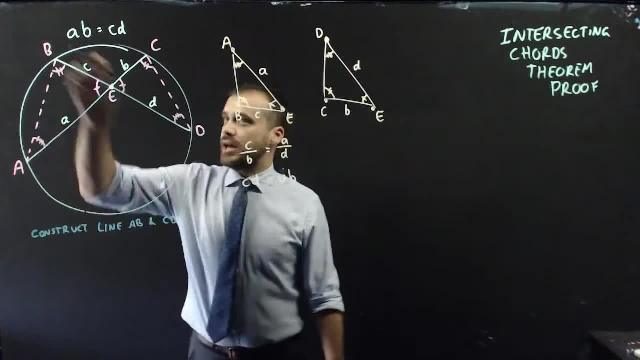 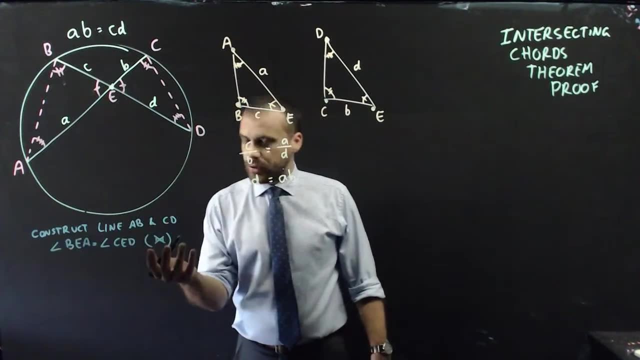 Alright, I'm just going to formalise it a little bit. First thing I did was construct line AB and line CD, so I'd have two triangles. Next I looked at those angles and saw that they were the same. They were the same because they were vertically opposite, so I aligned the two little angles in there. 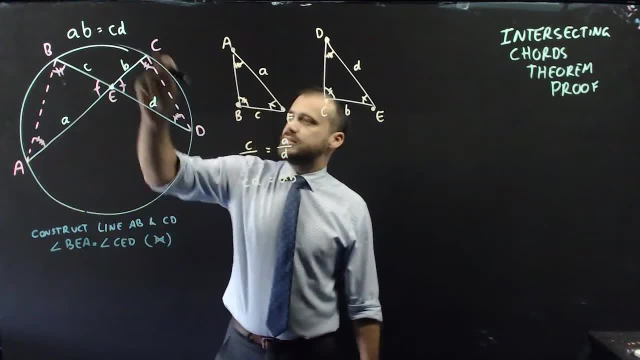 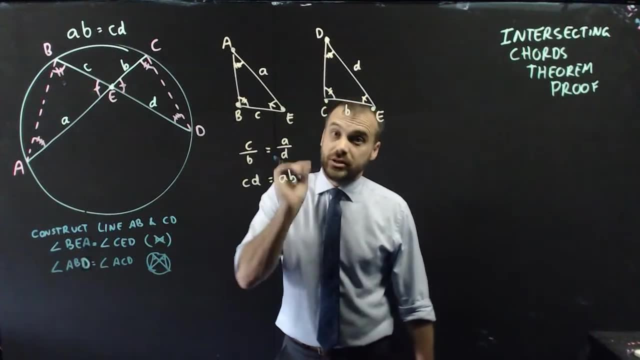 Okay, from there I can say that angle ABD and angle ACD were the same Because of this little bowtie here, or multiple mountain, or whatever you want to call this theorem here, angle sub 10. They ended off the same arc.